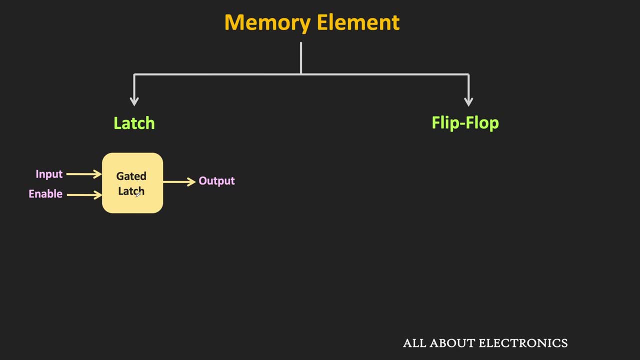 to that input change And in that case it retains its previous state. Now when we apply the periodic clock signal to this enable input, then the same gated latch can be used as the synchronous memory element. So this is the gated latch, Because now this latch will respond to the input when the clock signal is high. 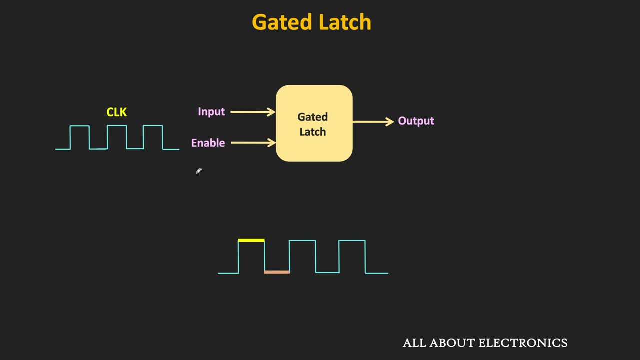 And it will remain in its previous state when this clock signal is low. So, as you can see, basically it is sensitive to the clock signal level, But during this on time of the clock, if the input level changes, then it will respond to that change immediately. 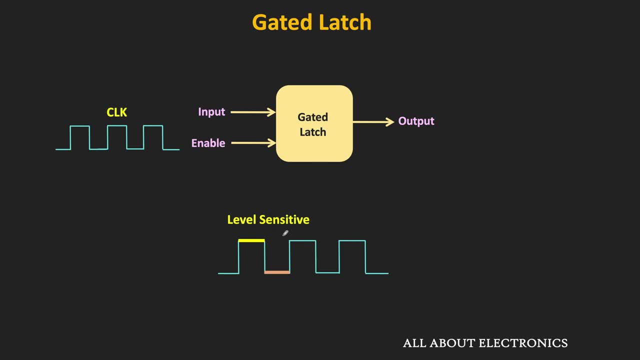 So let us understand the working of this gated latch with the help of the timing diagram. So let's see, Here we have one gated latch and the clock signal is applied as the enable input. So here the signal which is shown in the blue color is our clock signal. 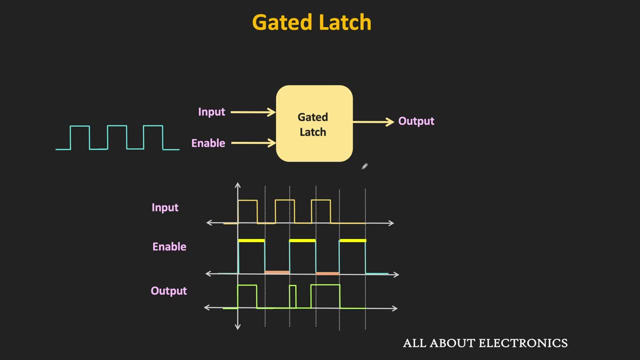 And that signal is applied at the enable input. So, as you know, this gated latch will become transparent when the clock signal is high, Or in other words, when this enable input is high. So, as you can see, during the on time of this clock signal, when the enable input is high. 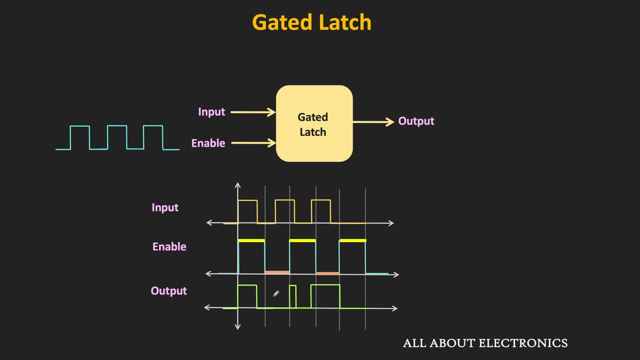 then the output is low And the output of the latch is same as the input signal. And after that, when this enable input becomes low, then even if the input signal changes, then also this latch will not respond to that input change. 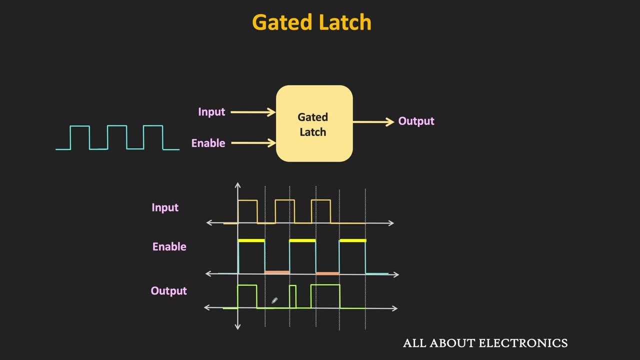 And, as you can see, it is retaining its previous state. So in this case, during the off time, it will remain zero. Now, once again, during the on time of the clock, when the enable input becomes high, then once again the output will follow the input signal. 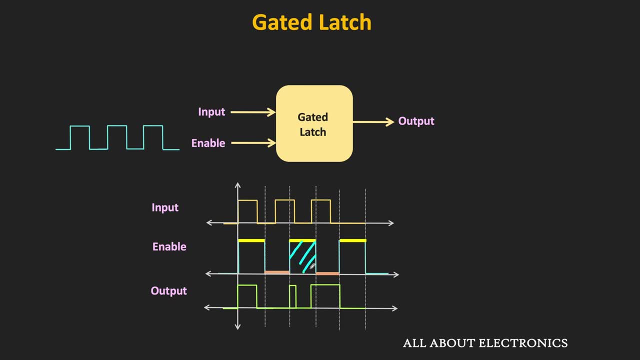 So, as you can see, during this time this output is following the input signal And, once again, during the off time of the clock signal, it will retain its previous state. So, as you can see, during this off time the input is going from high to low. 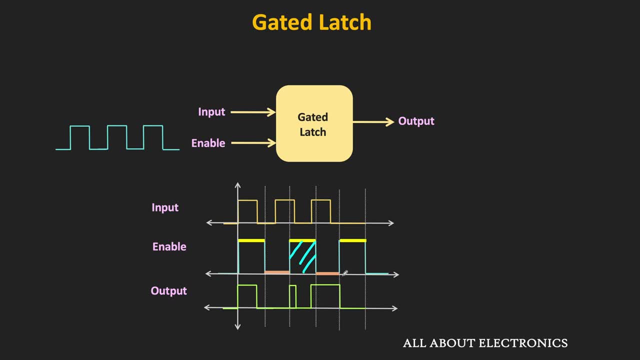 But still this latch will not respond to that input change And it will retain its previous state. Now, once again, it will become transparent to the input when the clock signal is high, Or in other words when the enable input becomes high. then also this latch will not respond. 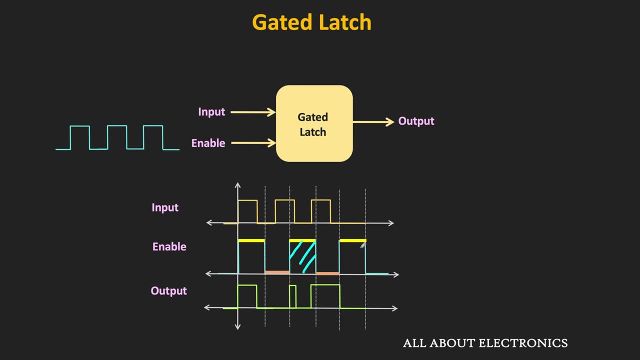 to that input signal, Or in other words, once again, when the enable input is high. So at that time, since the input is low, so the output will also become low. So this is the output of this gated latch. And, as you can see, when this periodic clock pulse is applied at the enable input, then 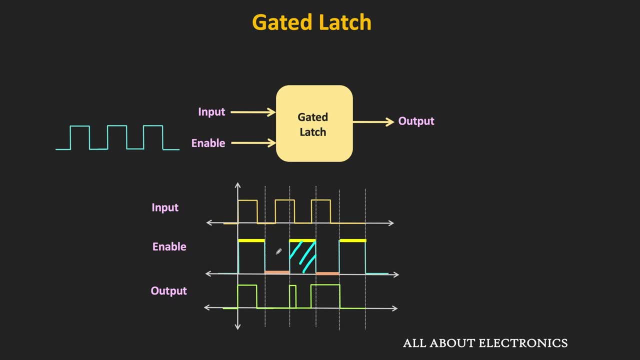 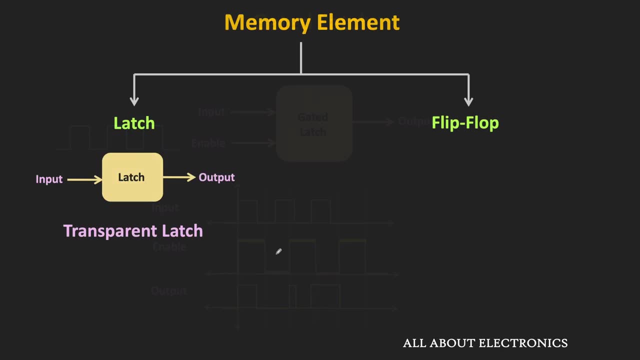 this gated latch will become level sensitive memory element. That means it will become transparent when this clock signal is high. On the other hand, if you see the flip-flop, then it also has clock input And it responds to the input only at the clock transition. 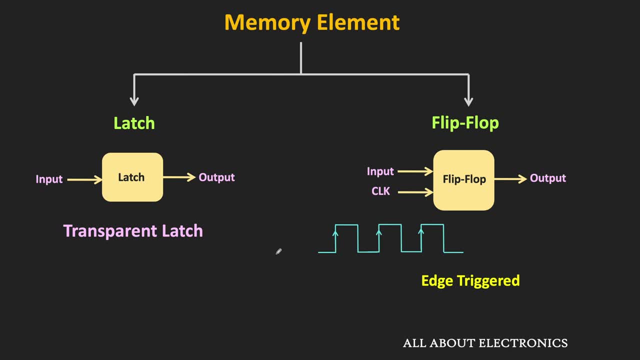 That means the flip-flop is the edge-triggered memory element. On the other hand, if you see the latch, then it is the level-triggered memory element. Now, this flip-flop can respond to the input either at the rising edge or the falling edge. 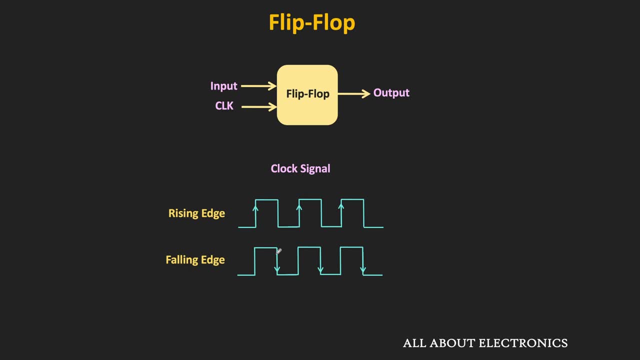 of the clock signal. So if it responds to the input at the rising edge, then it is called as the positive edge-triggered flip-flop. On the other hand, if it responds to the input at the falling edge of the clock, then it 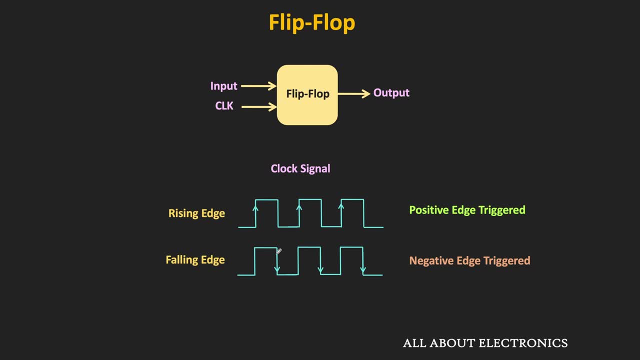 is called as the negative edge-triggered flip-flop. So through the timing diagram, let us understand how this edge-triggered flip-flop behaves to the input level changes. And first let us take the case of the positive edge-triggered flip-flop. 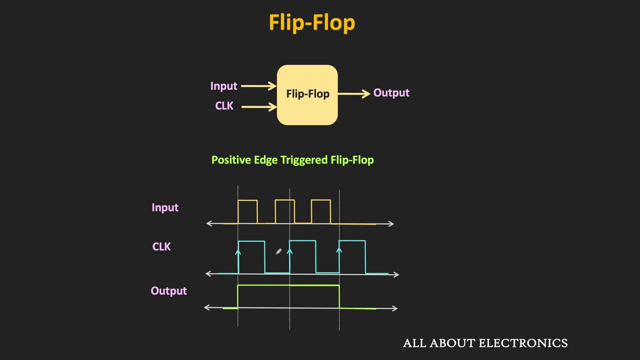 So here, the same signal which we have applied to the gated latch is also applied to the flip-flop, And this signal, which is shown in the blue color, is our clock. So since the flip-flop is the edge-triggered flip-flop, so it will respond to the input. 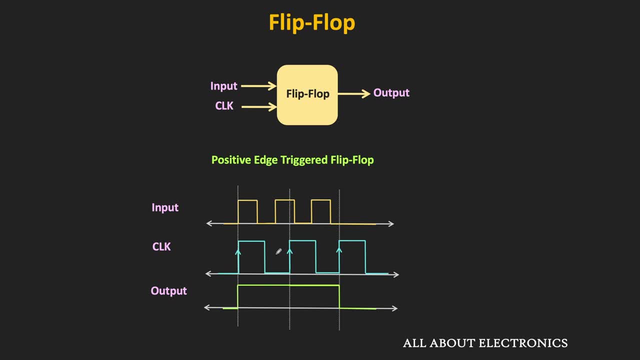 at the rising edge of the clock. And here we are assuming that at the clock transition the flip-flop follows the input signal. That means, at the clock transition if the input is high, then the output of the flip-flop is also high. 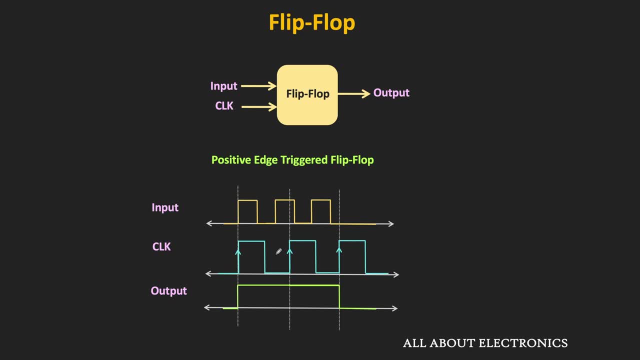 And if the input is low, then the output of the flip-flop will also become low. So, based on that assumption, let us see what will be the output of this clock. So, as you can see, at the first rising edge the input is high. 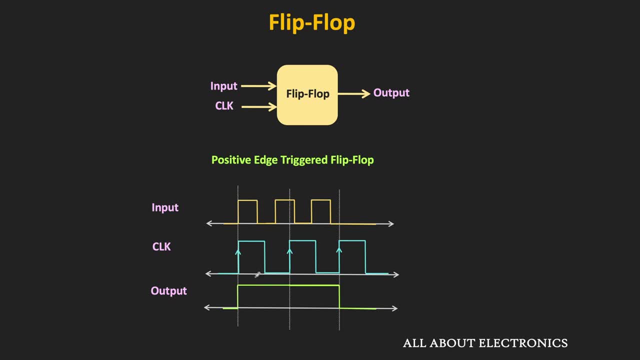 That means the output will also become High. But now the flip-flop will respond to the input at the next rising edge And till that it will retain its previous stage. That means in this case, until the next rising edge it will remain high. 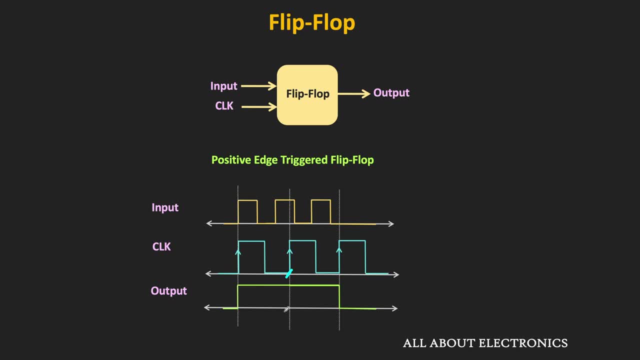 That means up to this point the output of the flip-flop will remain high. Now once again, at the next rising edge, rising gauge, the input is once again high. That means during the next clock transition also, the output will remain high. 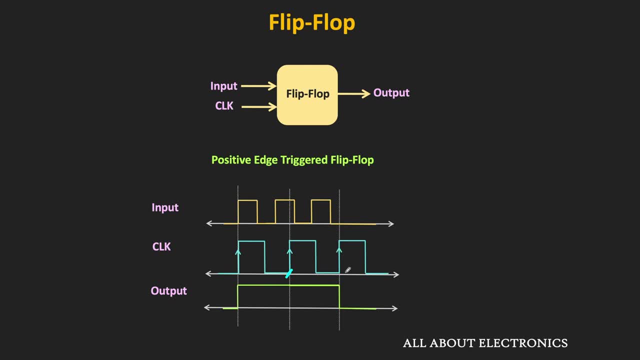 And it will remain high until the next clock transition. So in between, even if the input level changes, then also it will not respond to that input level change. So now at the next clock transition, since the input becomes low, so the output will. 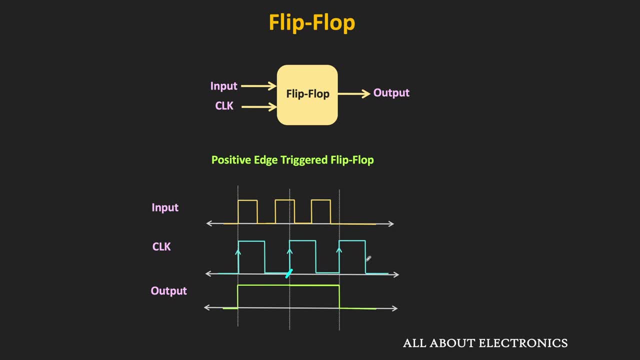 also become low, And it will remain low till the next clock transition. So, as you can see, this is the output of this positive, edge-triggered flip-flop. Similarly, for the same inputs, let's see the output of this negative, edge-triggered. 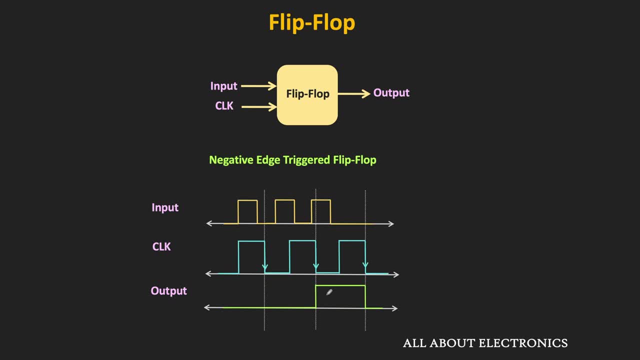 flip-flop. So this negative edge-triggered flip-flop will respond to the input at the falling gauge. So till the first falling gauge, the output of the flip-flop will remain zero. Now, at the first falling gauge, if you see. 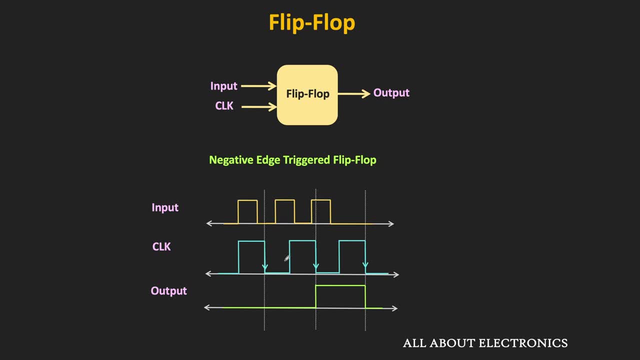 Then the input is low. That means the output of the flip-flop will also remain low, And it will remain in this state until the next falling gauge. Now once again at the next falling gauge, if you see, then the input becomes high. 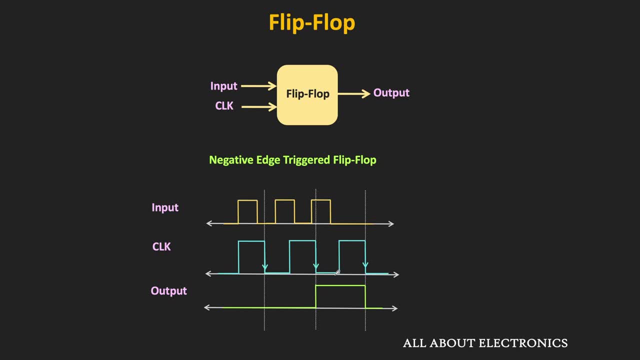 So since the input is high, so the output will also become high And it will remain in this state until the next falling gauge. So in between the two falling gauges, even if the input level changes, then also this flip-flop will not respond to that input level change. 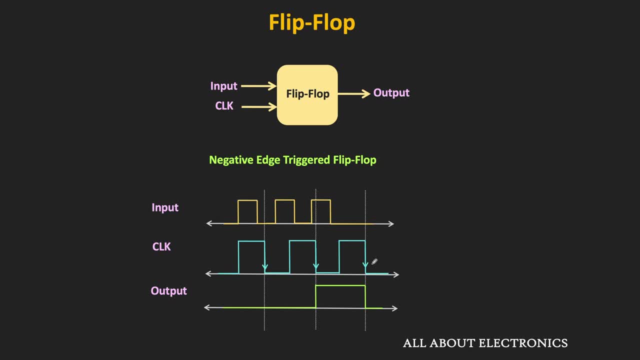 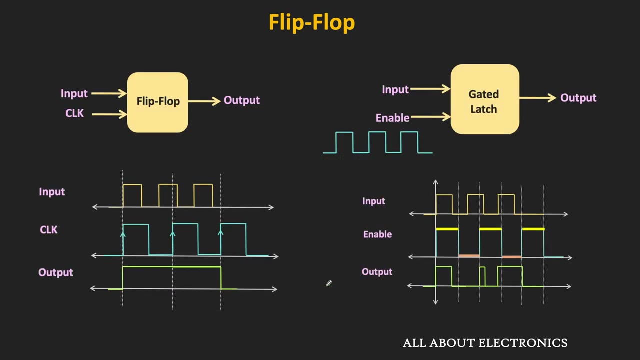 And at the next clock transition. if you see, then the input becomes low. That means now the output of the flip-flop will also become low. So overall this is the output of this negative edge-triggered flip-flop. So, as you can see, for the same input and the clock signal, the gated latch and the